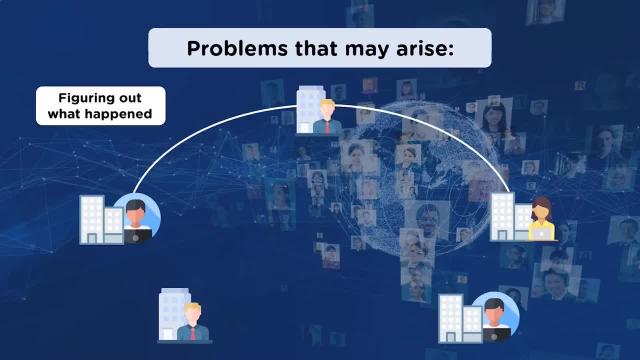 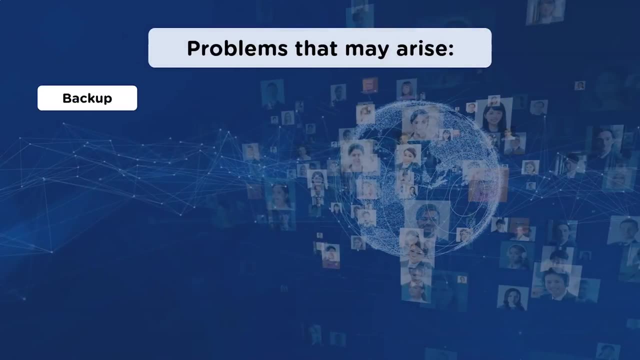 One more common challenge is to figure out what happened. At times, it is critical to know what changes are made to the previous version of the source code, if it is a verifiable, Or where exactly has the changes been made in a file. Then comes the problem of backup. 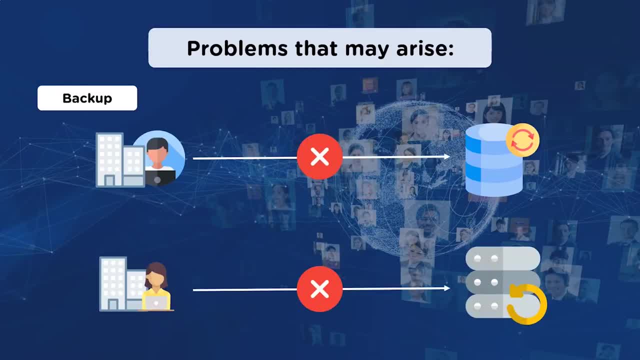 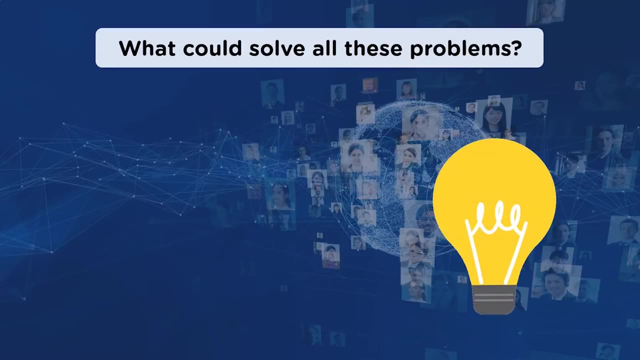 In case the system or the disk of the user breaks down and there is no backup, then all the efforts will go in vain. These are some of the basic problems that any small or big company might encounter. Now the question arises: what could be a possible solution to all such problems? 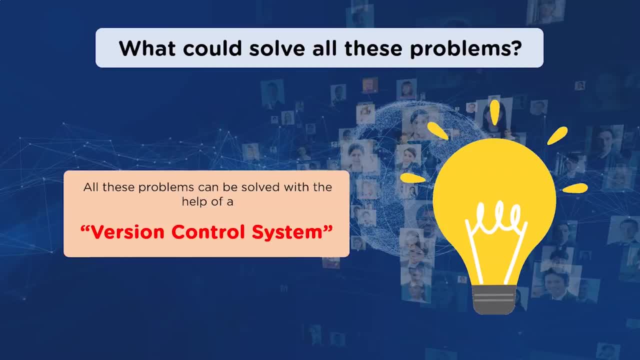 And this is when the version control system comes into picture. The version control system will take care of the collaboration between employees. Storing different versions will help in having backups on the remote repository. It will also help in rolling back to the previous commits and to the last version of the source. 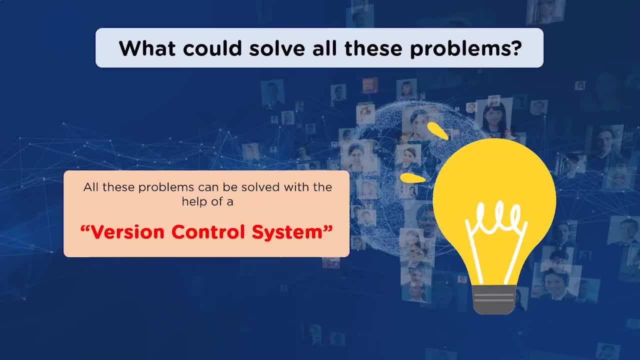 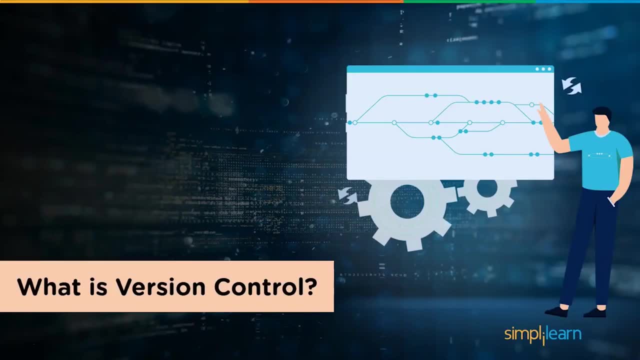 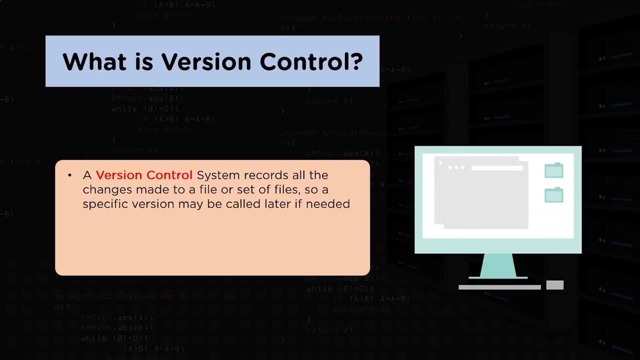 code. We will talk about each of these reasons in detail when we learn the benefits of the version control system. Let's first have a look at the version control system. First we will look at what is version control. As the name, version control, suggests, it refers to the category of software tools that make 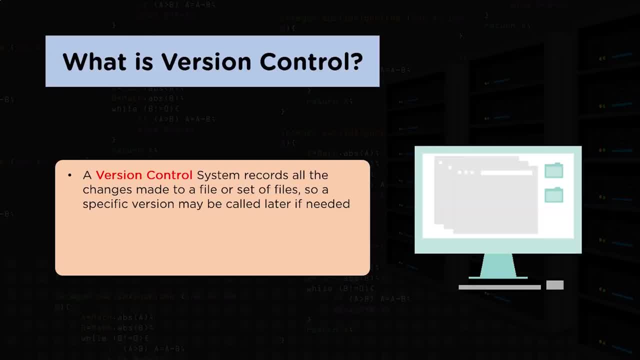 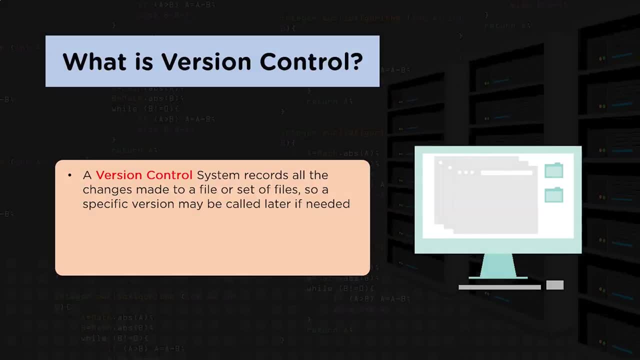 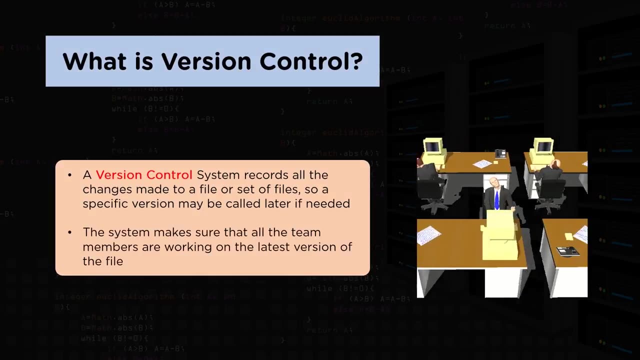 it possible for the software team to look after the changes made to the source code. The system records all the made changes to a file, so a specific version may be rolled if needed in future. It is the responsibility of the version control system to keep all the team members on the. 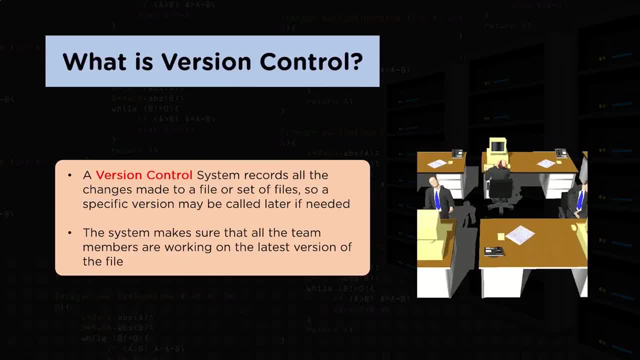 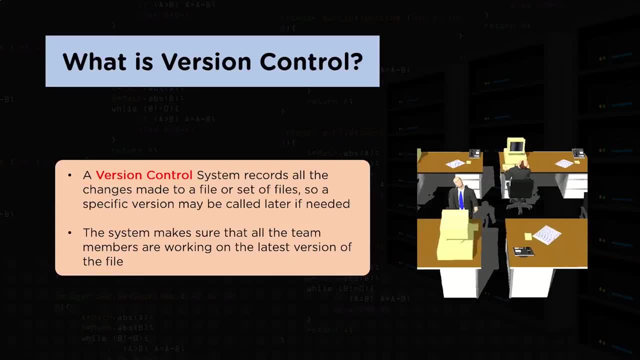 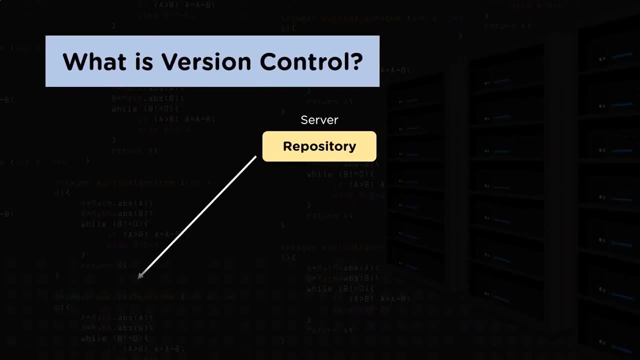 same page. It makes sure that every version is rolled, It makes sure that everyone on the team is working on the latest version of the files and, most importantly, makes sure that all these people can work simultaneously on the same project. Let's try to understand the process with the help of this picture. 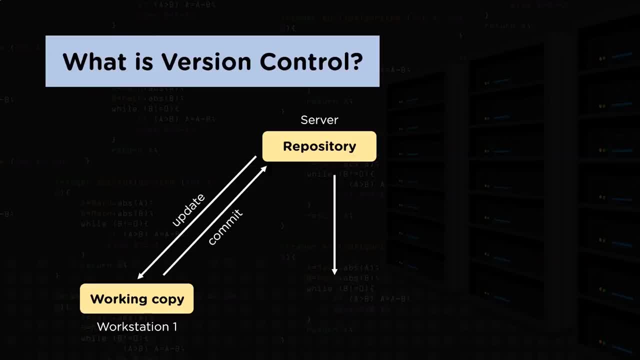 There are three workstations or three different developers, at three different locations And there is one repository that is acting as a server. The workstations are using the repository either for the process of committing or updating the tasks. There may be a larger number of workstations using a single server repository. 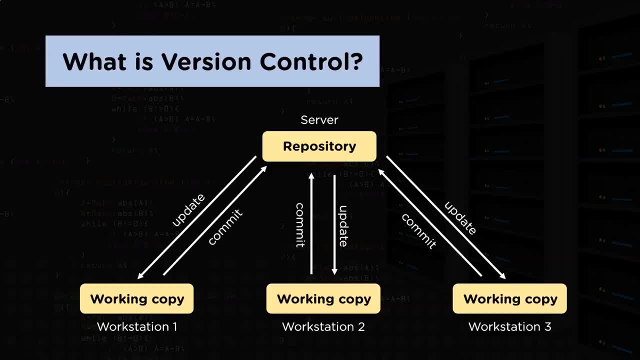 Each workstation will have its own working copy and all these workstations will be saving their source codes into a particular server repository. This makes it easy for any developer to access the task being done using the repository. In case the system of any particular developer breaks down, then also the work won't stop. 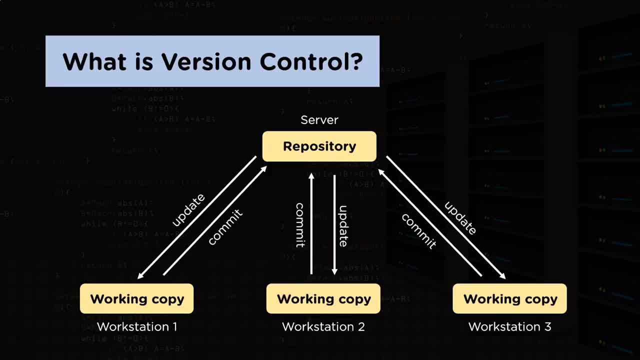 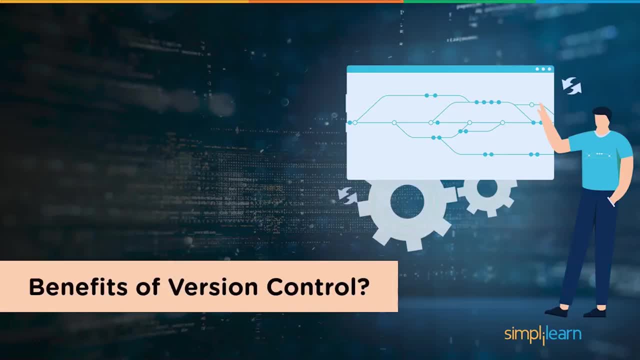 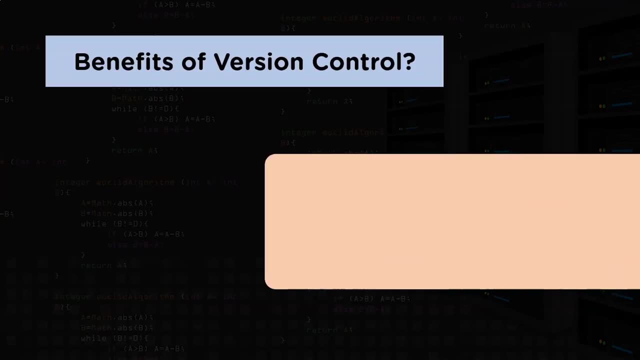 as there will be a copy of the source code in the central repository. Now, after knowing the basics of version control, it's time for us to check the benefits of version control. The first and the foremost advantage of the version control system is that it helps in 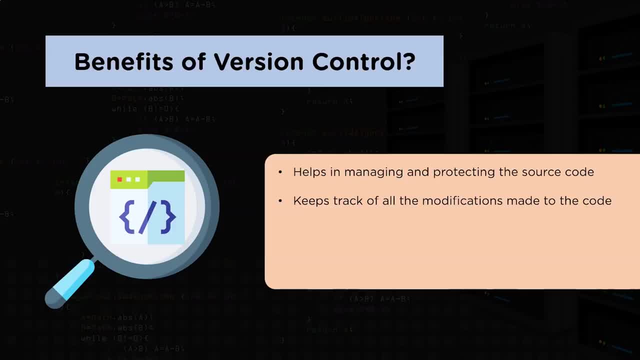 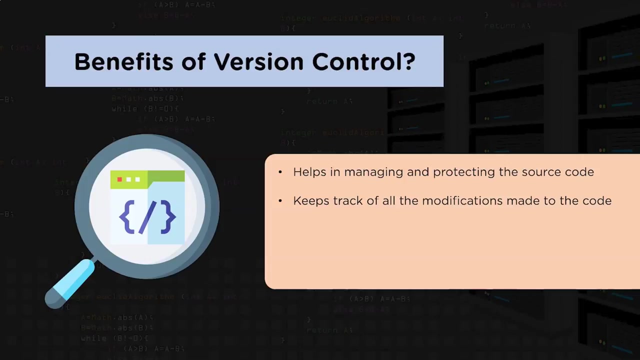 managing and protecting the source code. The system helps in management of the source code for the software team. by keeping track of all the modifications that are being made to the code, It also protects the source code from any unintended human error and consequences. Then the next advantage is it keeps record of all the modifications made to the code. 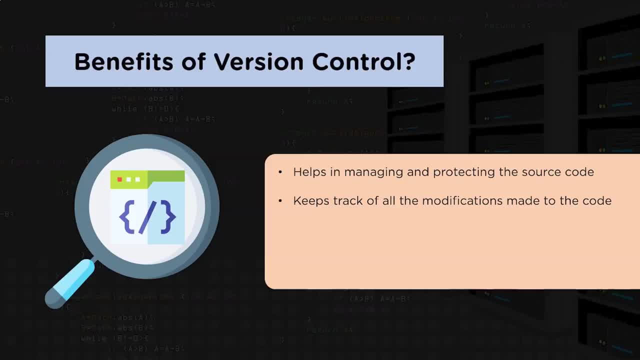 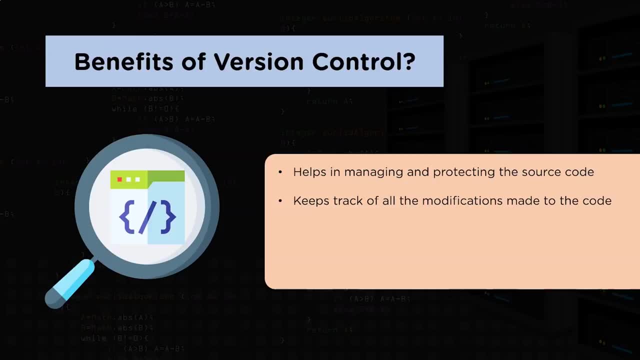 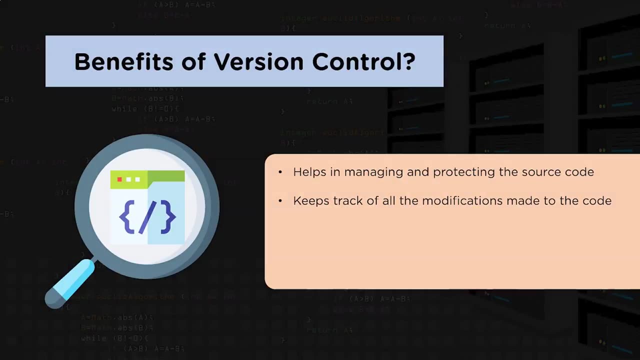 As we learned in the previous step, the way it manages the code for the software team. The team is working continuously producing new source codes and it is making amendments to the already existing code. These changes are to be recorded for future references And in case they are needed, to discover the root cause of any particular problem. 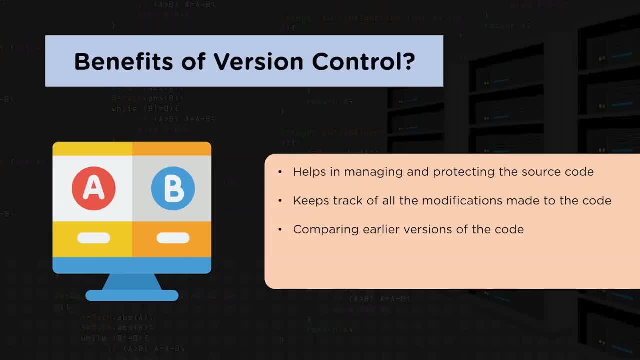 Then the third advantage here talks about comparing earlier versions of the code. As we saw that all the versions of the source code are saved, This makes it possible for developers to go back at any time and compare the earlier versions of the code to help fix the mistake, while reducing disruption to all team members. 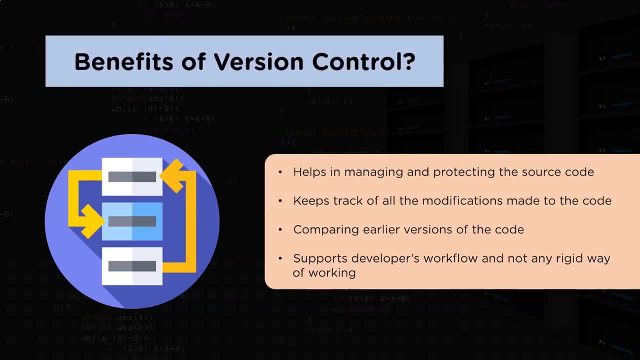 The fourth and the final benefit of the version control system is that it helps in managing all the changes made to the code. The third and the final benefit we shall see is that the version control system supports developers workflow and not any rigid way of working. 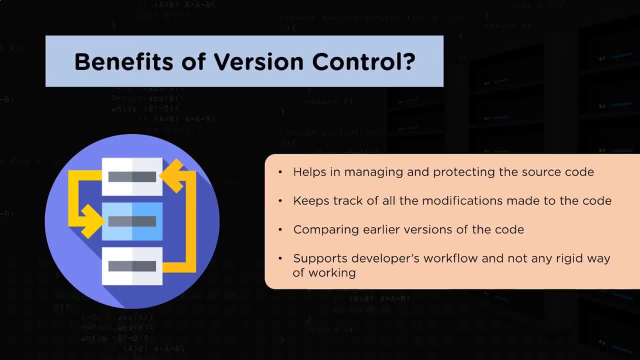 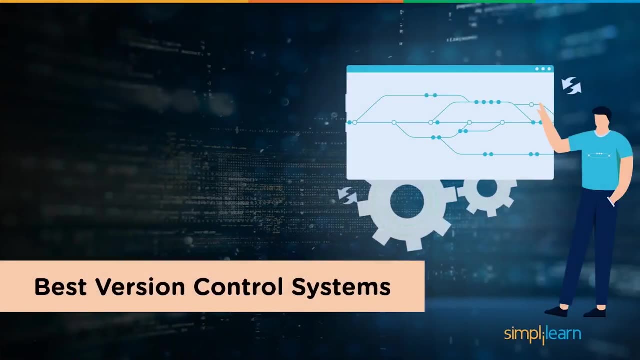 Any good version control system will not impose any particular way of working. The version control systems are known to provide smooth, continuous flow of changes made to the code and prevent developers from getting frustrated in the course of this mechanism. Now, towards the end of the video.